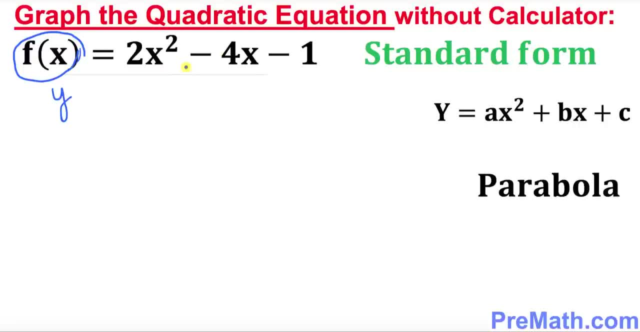 thing I want you to just keep in your mind that this equation, this quadratic equation, is in a standard form. So we will be dealing with standard form this time. So you might be wondering: what is the standard form? Standard form is, of this form, y equal to. 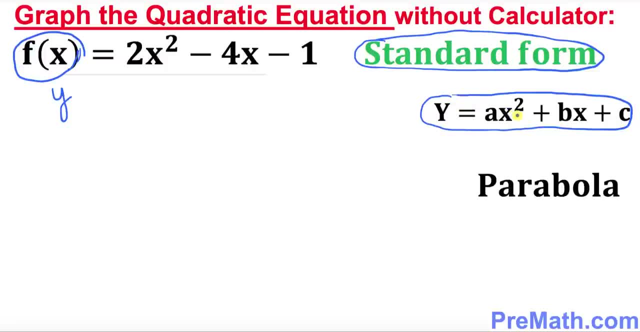 a- y equal to a, x squared plus b, x plus c. This form is called standard form. And finally, these kind of quadratic equations are also called parabolas. So parabola is of this kind of shape: Okay, if it opens up it looks like this kind of shape. Okay, It is this kind. 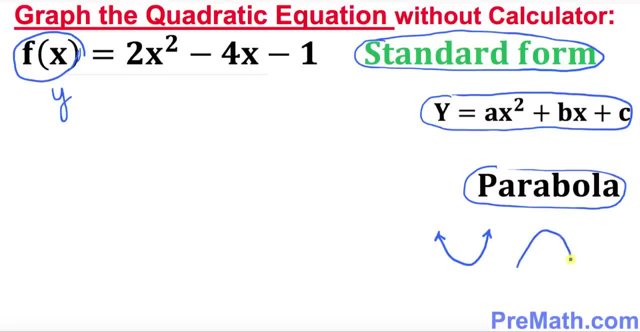 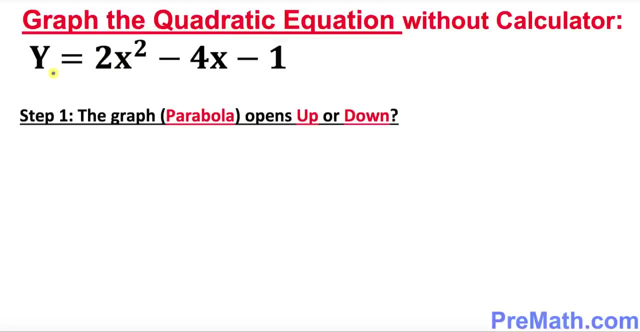 of graph And if it opens down, it looks like this. So this duda again looks like this kind of graph. We're going to go over, step by step, the entire process, so let's see what happens. So in the very first step, we have this quadratic equation in a standard form. Let's find out. 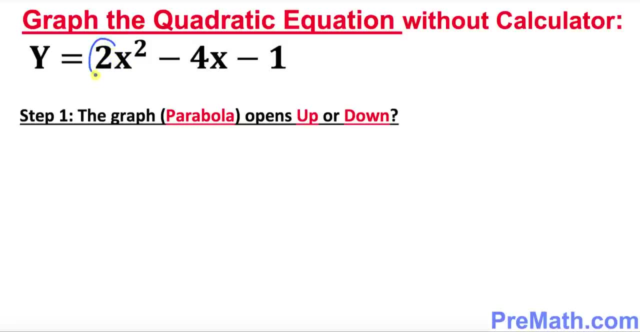 what is our a, b and c In this case? this is our a, this is our b and this is our what c? So a equals to how much 1…0.Missed 1…0.. In this case, it looks like this kind of graph: 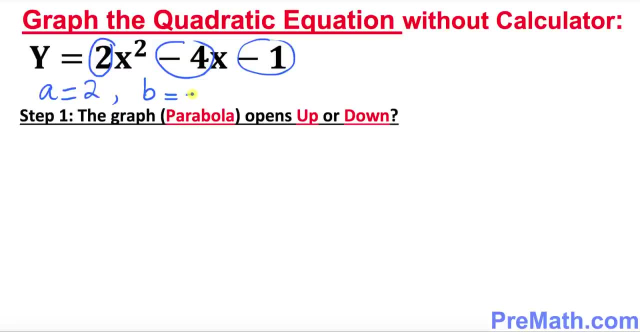 much: 2, b equals to negative 4 and c equals to negative 1.. So the very first step is asking this graph, which is also called parabola, does it open up or opens down? So always check at your a. If a is c over- here is your leading coefficient- is positive, then it's going to open up. So the 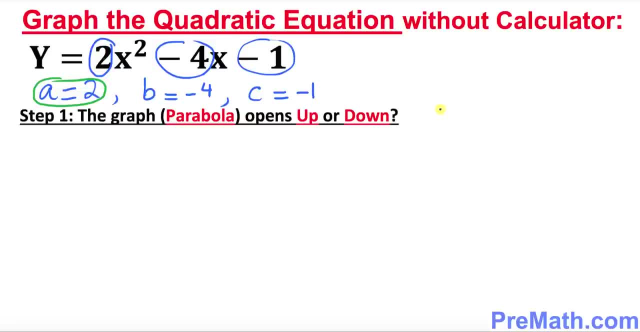 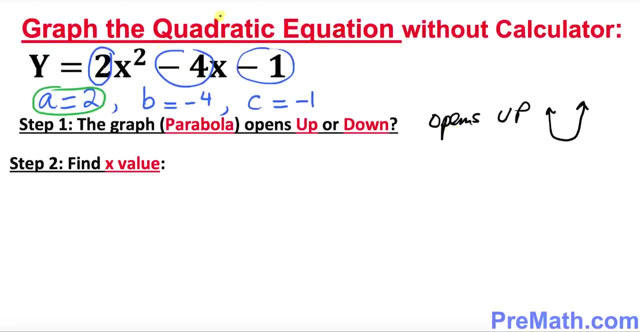 very first thing, I want to make sure that this opens up. That means this is going to look like this kind of graph. In the second step, we want to find x value. So what is the x value is going to be This one over here? This is the formula you have to put down: x equals to minus b over what? 2a. 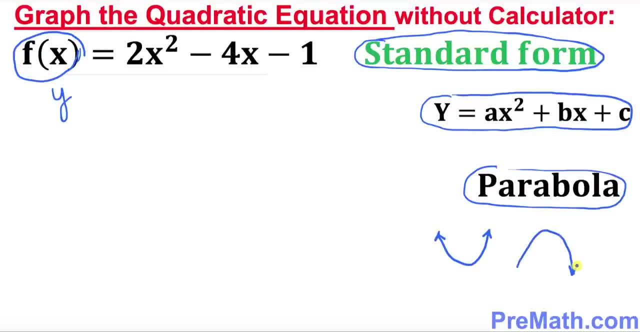 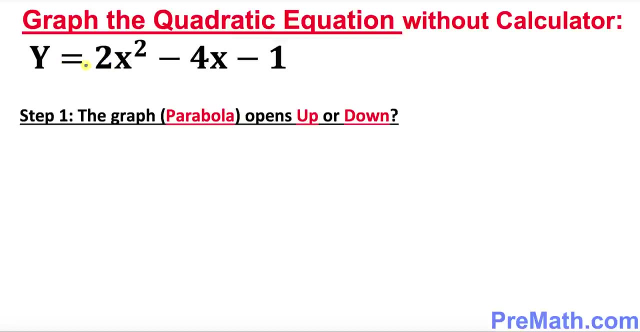 if it opens down, it looks like this. So this is the standard form. And finally, these kind of quadratic equations are also like this kind of graph. We are going to go over step by step process, So let's see what happens. So in the very first step, we have this quadratic equation in a standard form. Let's find out. 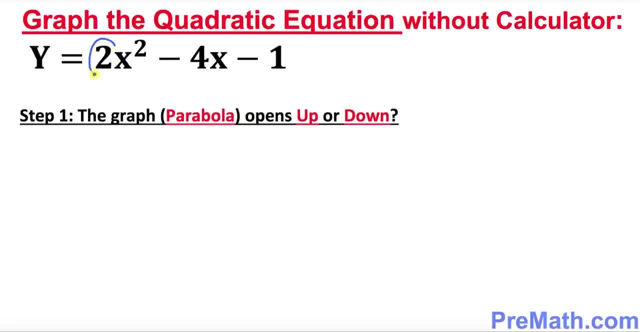 what is our a, b and c In this case? this is our a, this is our b and this is our what c. So a equals to how much 2, b equals to negative 4 and c equals to negative 1.. So the very first step is asking: 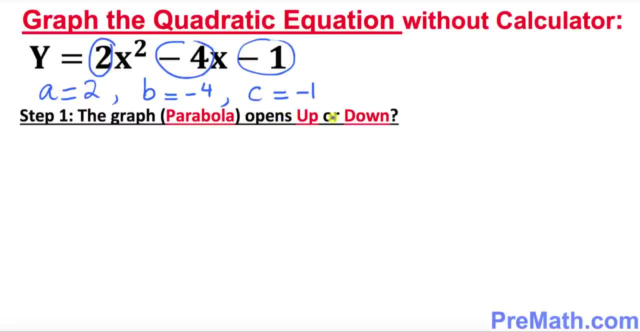 this graph, which is also called parabola, does it open up or opens down? So always check at your a. If a is see over here- is your leading coefficient is positive, then it's going to open up. So the very first thing I want to make sure that this opens up. That means that this is: 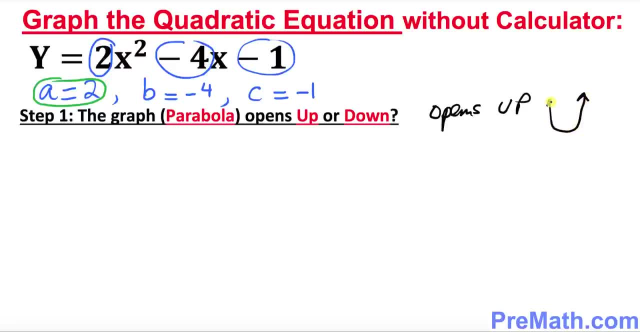 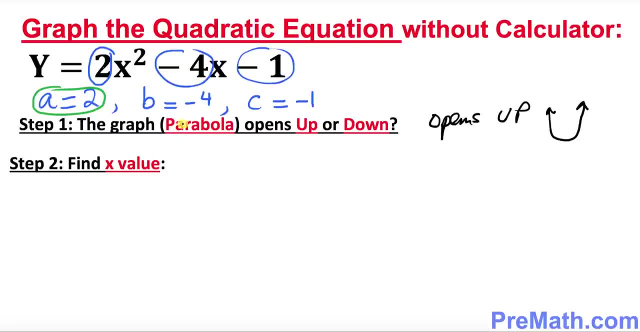 going to look like this kind of graph. In the second step, we want to find x value. So what is the x value? It's going to be this one over here. This is the formula you have to put down: x equals to minus b. over what? 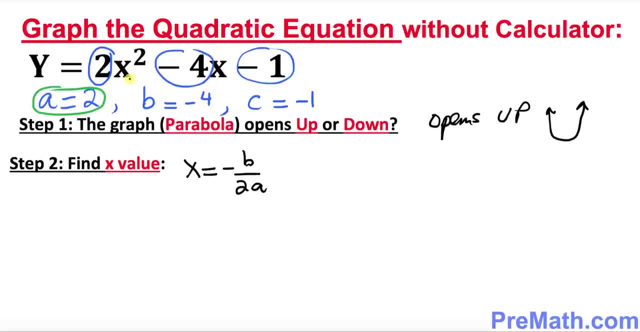 to a, so in our case b is negative 4, a is 2, so that's going to give us how much. so that means it's going to be x equal to minus and b is negative. 4 divided by 2 times a is 2, so negative. 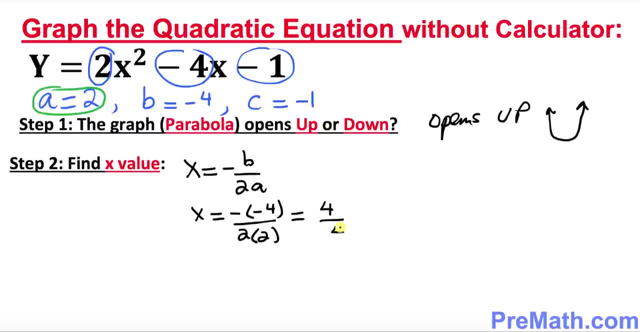 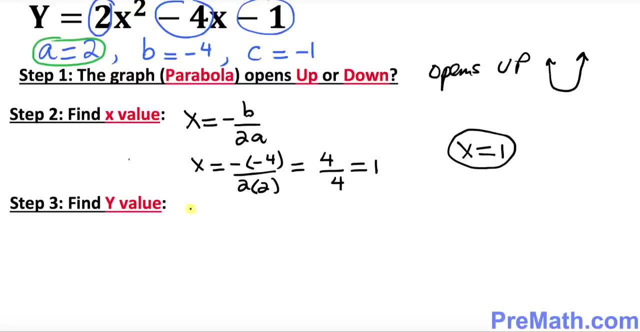 and negative become positive. 4 over 4, that is equal to 1. so that means thus our x value turns out to be 1. in step number 3, we want to find y value. so what we're going to do is look at your original equation. we have y equals to 2x square. so wherever you see x, you replace it by this. 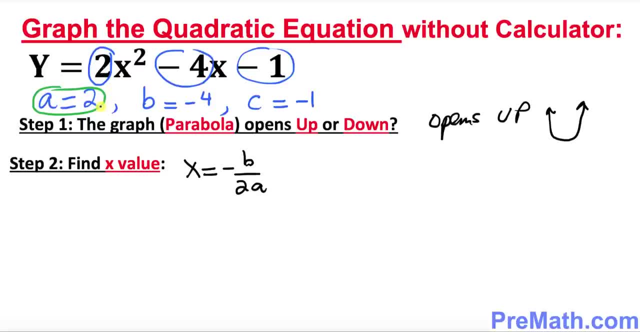 So in our case, b is negative, 4, a is 2.. So that's going to give us how much. So that means it's going to be x equal to minus and b is negative. 4 divided by 2 times a is 2.. So negative and negative. 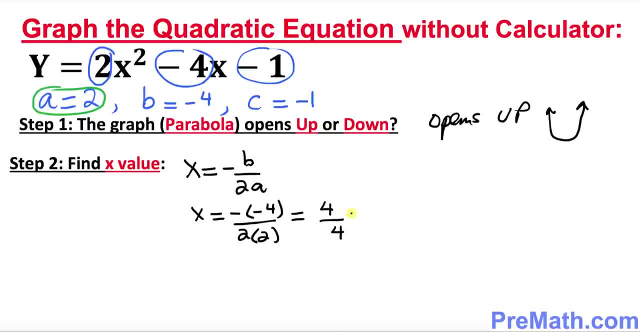 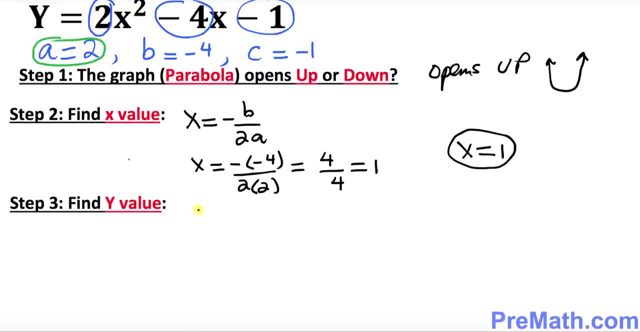 become positive, So that's going to be positive. 4 over 4, that is equal to 1.. So that means thus our x value turns out to be 1.. In step number 3, we want to find y value. So what we're going to do is look at your original. 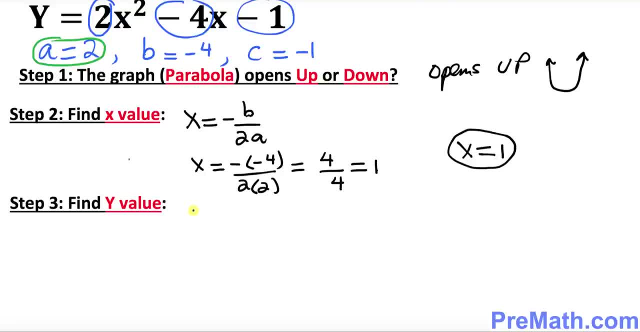 equation We have y equals to 2x squared. So wherever you see x, you replace it by this 1 that we found, We found out. second step. So this: when we plug it in, x equal to 1.. So y equals to how much 2 times. 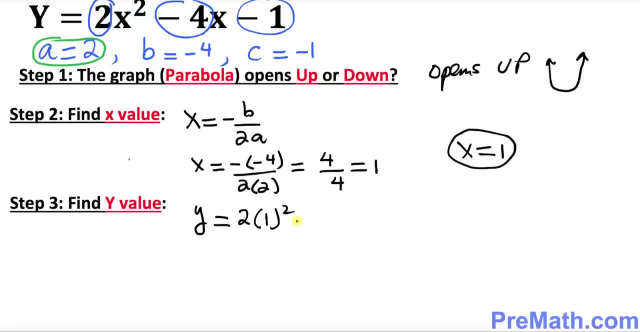 1 squared minus 4 times 1 minus 1 in our original equation. So this is going to become: 2 times 1, squared is simply: 1 minus 4 times 1 is 4.. And then negative. So that's going to give you how much 2 minus 4 minus 1.. So that's going to give you how much. 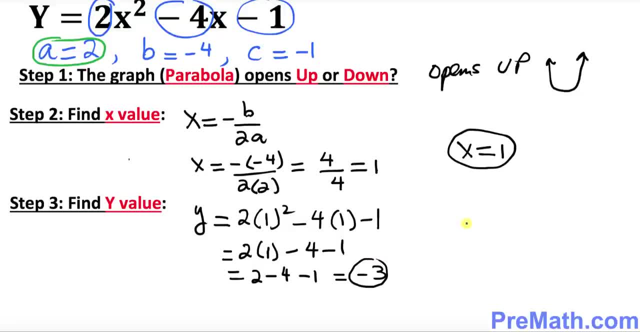 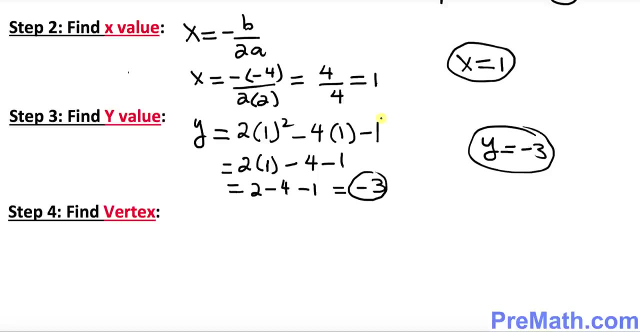 Negative 3. So that's that means. so your y values turns out to be what Negative 3.. In step 4 now we want to find the vertex. So vertex- always remember vertex- is simply your x and y values are called vertex. So in this case, in our case, we already figured out x value. 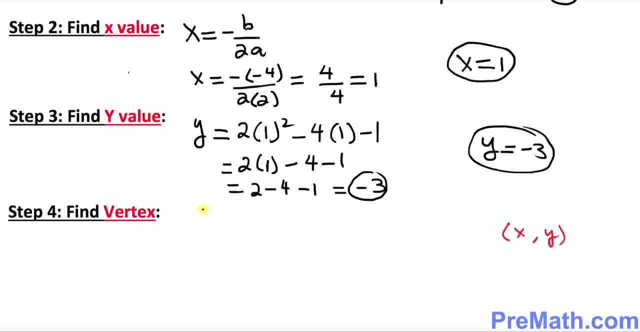 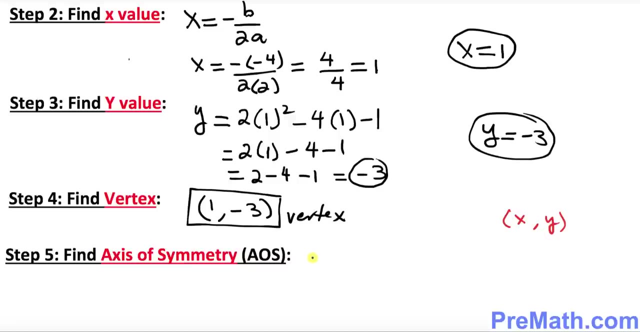 and y value. that's you just going to be. So our vertex is going to be. is simply what? 1 comma negative 3.. So that is our vertex. In step 5, we want to figure out the x's of space. So we're going to find the x's of space, So that's. 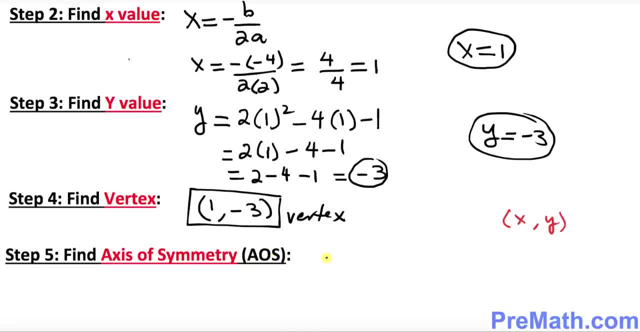 what we're going to going to find. We need to find the x's of space, All the x's of space. children in this block can come from various daunting problems And the ticket plus points is going to be x's of space. So we need to first snap in the x's of place And that's b is a constant value of x equal to 1. 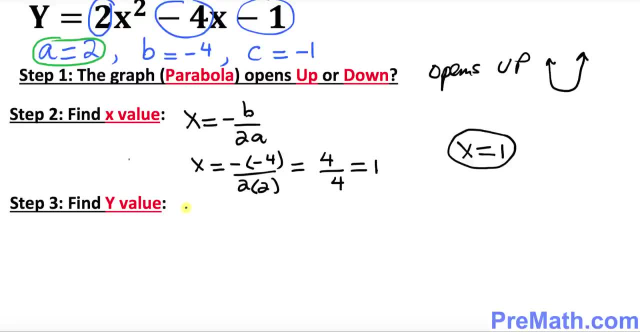 1 that we found out. second step. so this is when we plug it in: x equal to 1, so y equals to how much 2 times 1 square minus 4 times 1 minus 1 in our original original equation. so this is going to: 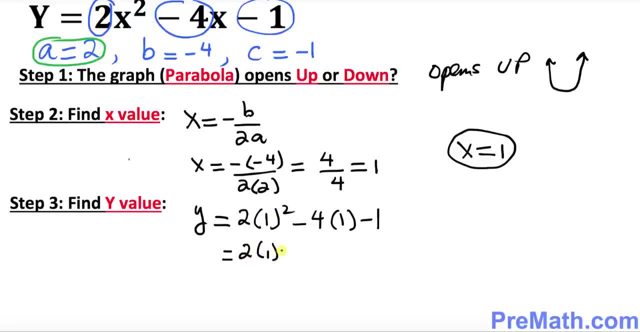 become 2 times 1. squared is simply 1 minus 4. times 1 is 4, and then negative 1. so that's going to give you how much 2 minus 4 minus 1. so that's going to give you how much negative 3. so that's, that means. 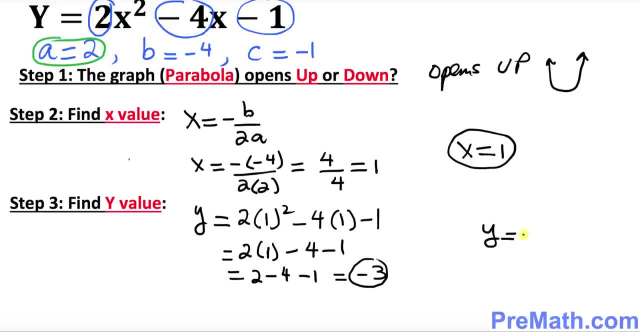 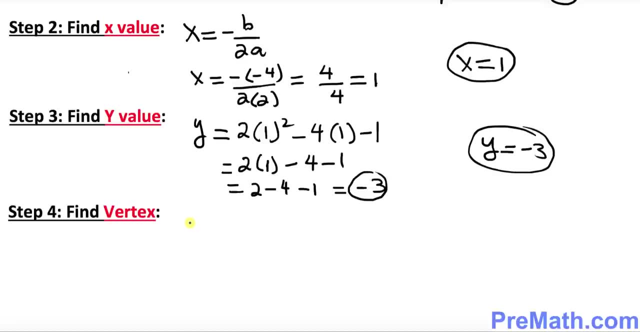 so your y values turns out to be what negative 3. so in step 4 now we want to find the vertex. so vertex, always remember, vertex is simply your x and y values are called vertex. so in this case, in our case, we already figured out x value and y value. 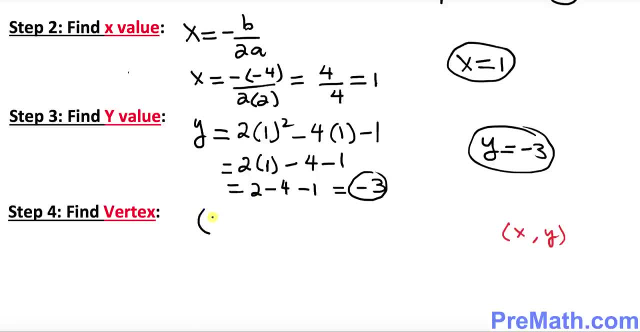 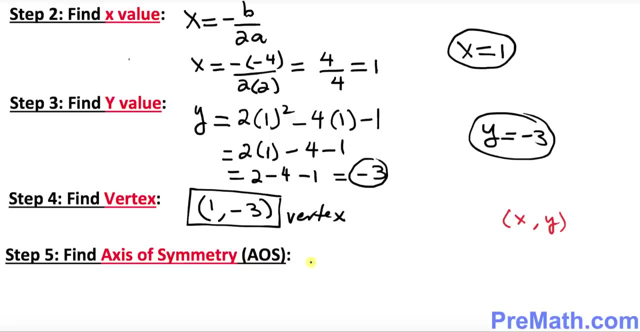 that's you just going to be. so our vertex is going to be simply what? 1 comma negative 3. so that is our vertex. in step 5 we want to figure out the xs of symmetry, or we simply call it AOS. so x of symmetry is simply always. 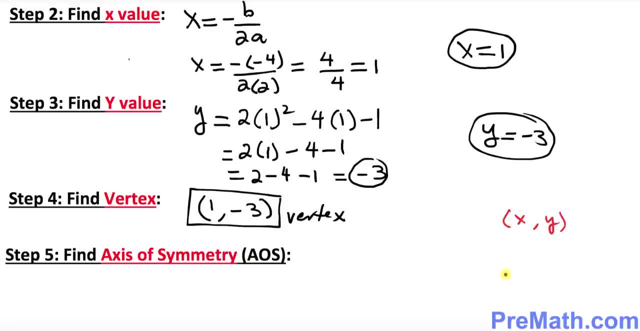 remember, x of symmetry is: AOS is always you have something x equal to some value, so that is your x of symmetry. in our case, then it's going to be simply whatever we call it here, say x and y, but this mod then has to be equal to a, 2 and 1.. 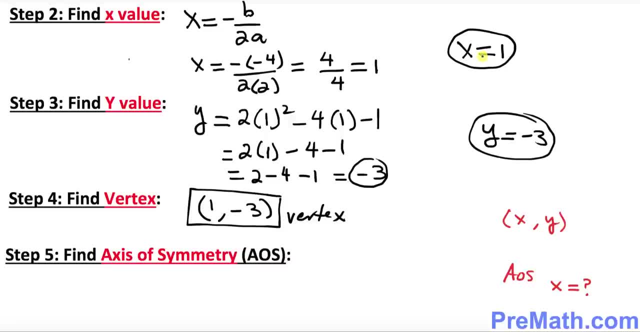 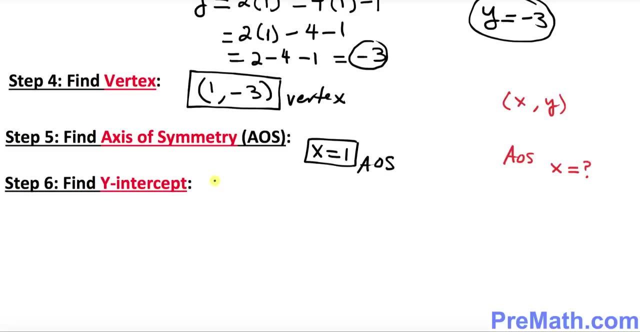 case, then it's going to be simply whatever we got in step two, this x value, that's going to be our axis symmetry. So x equal to 1 is our axis of symmetry. In step six we want to figure out y intercept. that means the point on y axis. Always remember for a point on y axis or y intercept. 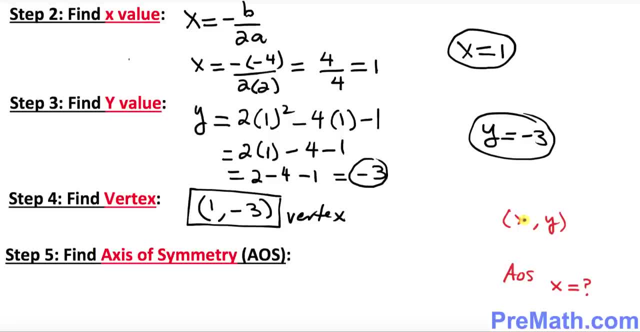 and well, 2 times q is a constant of x's of space. We are going to make thisis what I call this x's of space. so these are Buenos coughs and whoever: 12 x's of space in zy from wrong, goes to these 10x's of space. 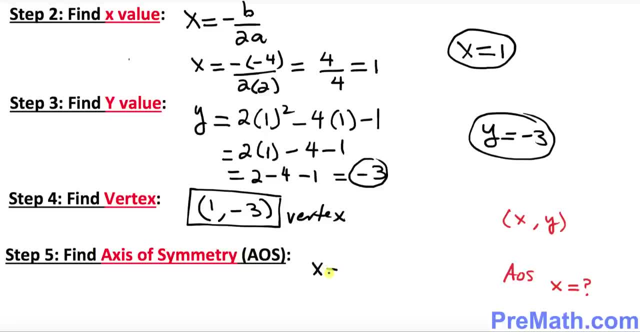 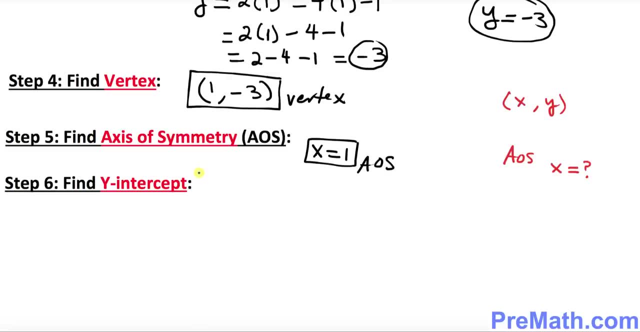 Why? Because you just宽 I'm going to cheer everybody out and add to it our x's of space right here where you go two times. So so every entry that we we come to is really to the left and we go down to to 1 is our axis of symmetry. in step 6 we want to figure out Y intercept, that 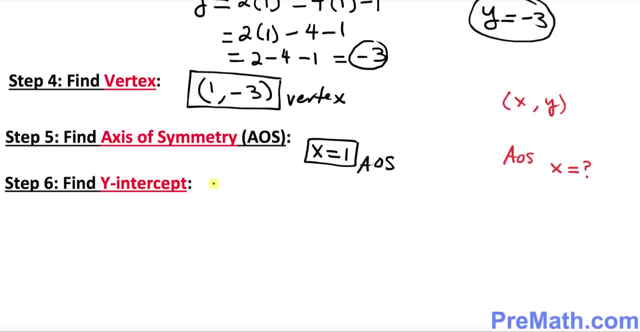 means the point on Y axis. always remember, for a point on Y axis or Y intercept, X is always equal to 0. so we say: put X equal to 0. so then in our original equation, what was that? one which is Y equals to 2x square minus 4x. 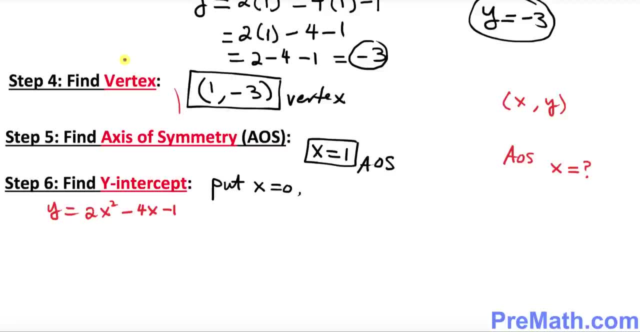 minus 1. so wherever you see X, replace it by 0. so this is going to become how much 2 times 0 square minus 4 times 0 minus 1. so this is going to become how much 2 times 0 square minus 4 times 0 minus 1. 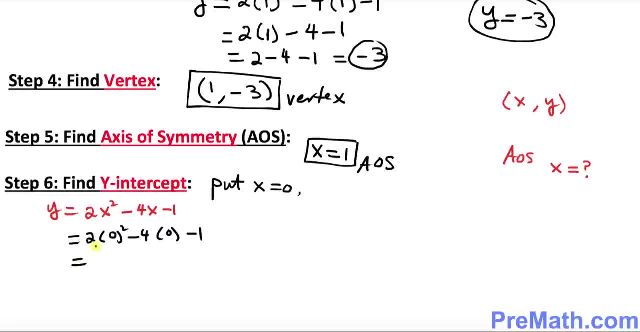 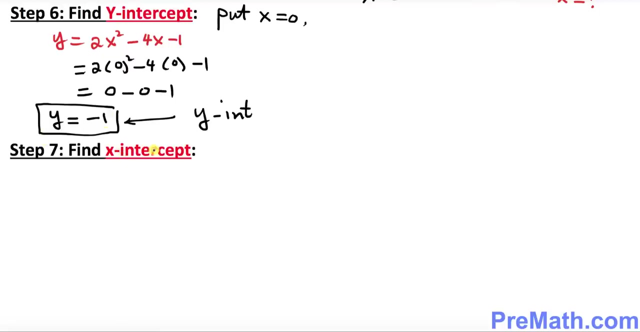 so that's going to be how much 0 times 2 is 0 minus 0 minus 1. so that means simply Y equals to how much negative 1. so that is our Y intercept. in step 7 we want to figure out X intercept. as you recall that to find X intercept we all 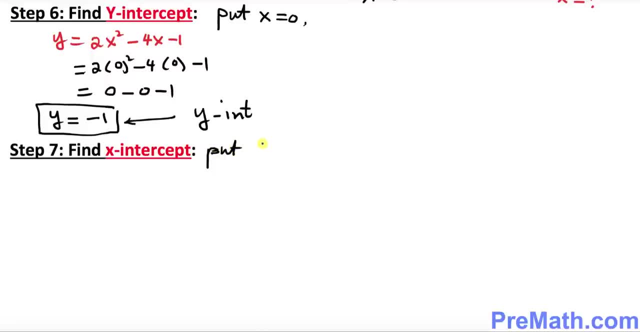 1. todasальmente colocar Y equal to how much? 0. so then, if Y equal equal to zero, our original equation, which is what Y equal 2x square minus 4x minus 1, wherever you see dancing Y will turn into 0. so then, 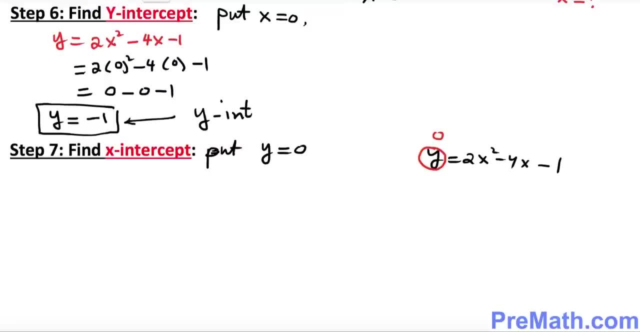 we können 0, we get what. so we got a quadratic equation when X equals 0 and in we ended up with what a quadratic equation. when X equals 1, we had 2, 40 going on. y equals 2. you can get here what deliberate equation and this y is we need to. 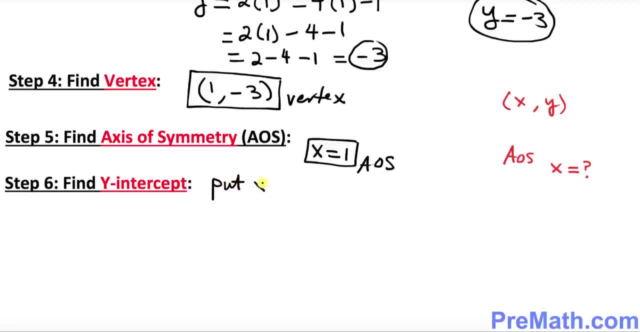 x is always equal to 0. So we say, put x equal to 0.. So then, in our original equation- what was that? one which is y equals to 2x square minus 4x minus 1.. So wherever you see x, replace it by 0. So this is going to become how much 2 times 0 square minus 4 times 0 minus 1.. So 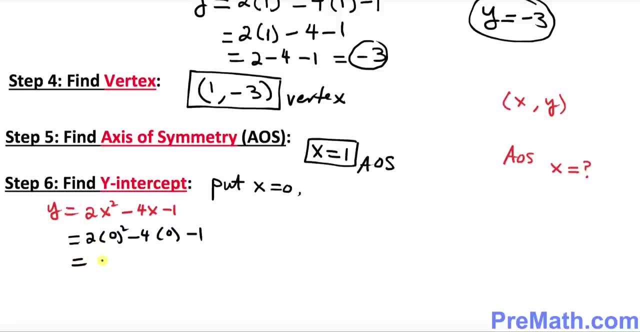 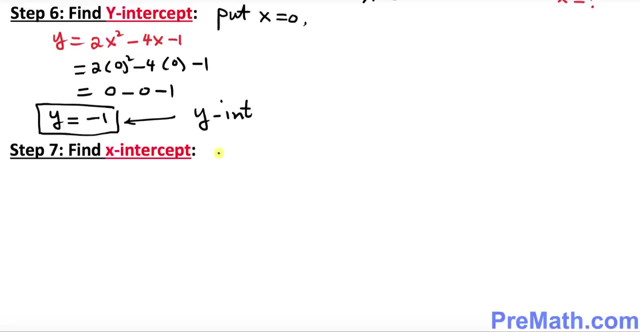 that's going to be how much 0 times 2 is 0 minus 0 minus 1.. So that means simply, y equals to how much Negative 1.. So that is our y intercept. Now let's get to step four. in step seven we want to figure out x intercept, as you recall that. 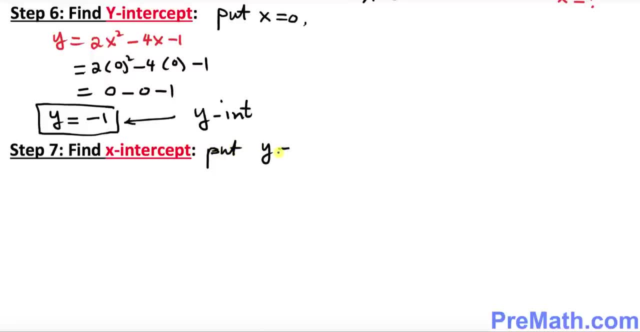 to find x intercept. we always put y equal to how much. we put y equal to 0.. Thus then, if y equal to 0, our original equation, which is what y equals to 2x square minus 4x minus 1.. 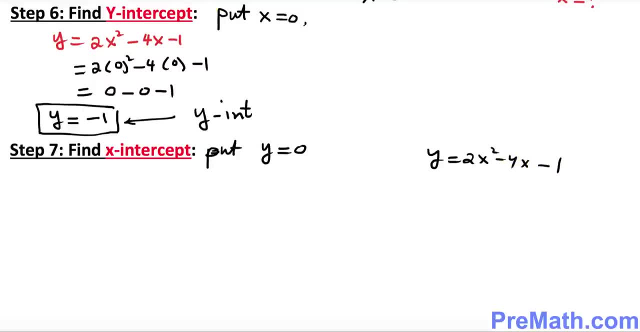 So, whatever way you see y equal to 0, because x is not equal to 0.う, Whatever way you see y equal to 0, the y equal to 0 is 2x to 3.. So what you see? x equal to x minus 4x minus 1.. 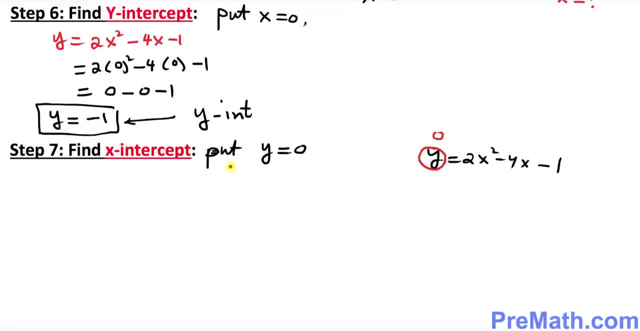 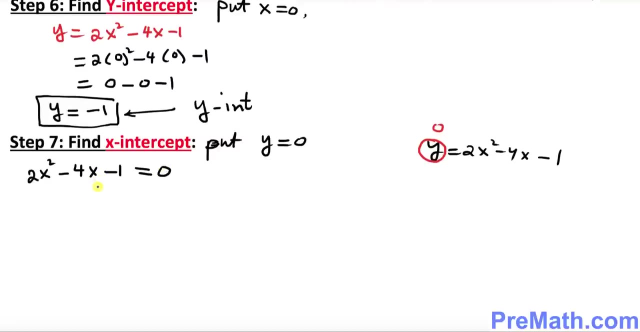 y. this y becomes what 0. So then we got what. So we ended up with what Quadratic equation: 2x square minus 4x minus 1, we set it equal to what 0. So now we have no option. 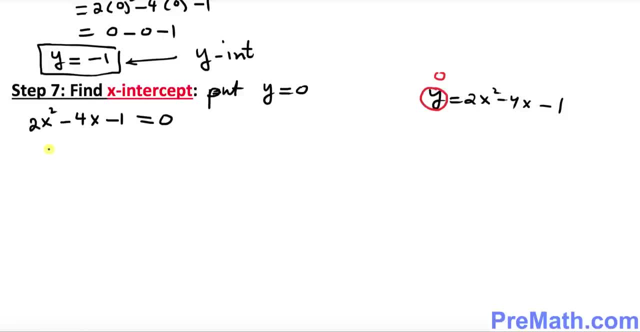 but to use a quadratic formula. So what is the quadratic formula? Quadratic formula: is x equal to minus b, plus or minus b square minus 4ac over 2a? So let's go ahead and solve using the quadratic formula. In our case, a equals to what? 2, b equals to negative, 4, c equals to. 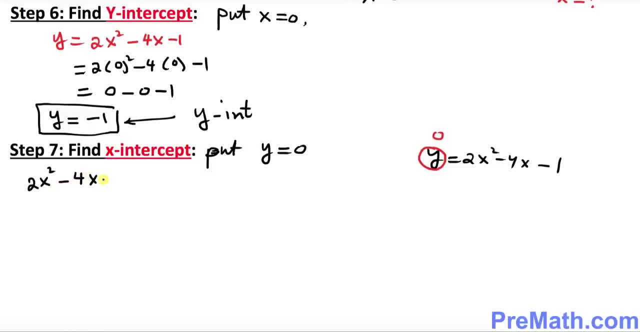 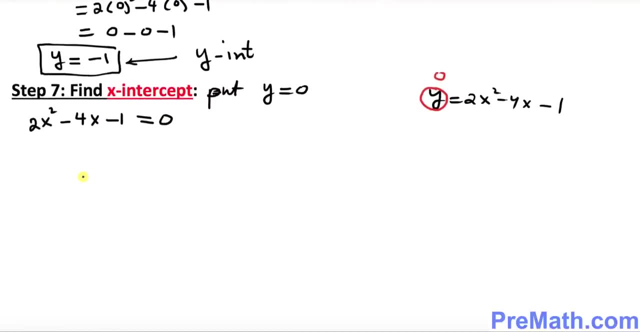 equation: 2x squared minus 4x minus 1, we set it equal to what? 0.. So now we have no option but to use a quadratic formula. So what is the quadratic formula? Quadratic formula is x equal to minus b, plus or minus b squared minus 4ac over 2a. So let's go ahead and solve using the. 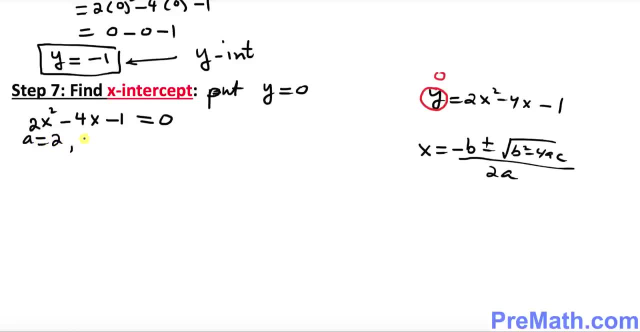 quadratic formula. In our case, a equals to what, 2b equals to negative 4, c equals to negative 1.. Let's plug it in in our quadratic formula to figure out x values. So x equal to minus and negative, 4b is negative. 4 plus minus b squared is going to be a negative 4 squared minus 4 times a. 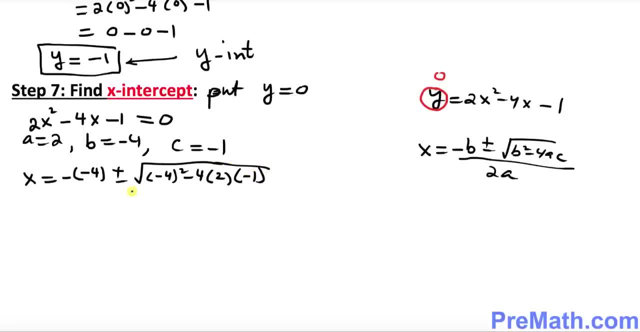 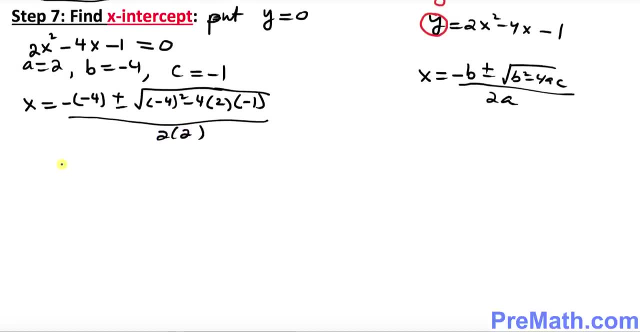 is 2 negative, 1. Everything Is divisible by 2 times 2.. So let's go ahead and simplify that thing. So x equal to what? 4 plus or minus 16 plus 8 divided by 4.. Let's simplify: 4 plus or minus square root of 24 divided by 4.. 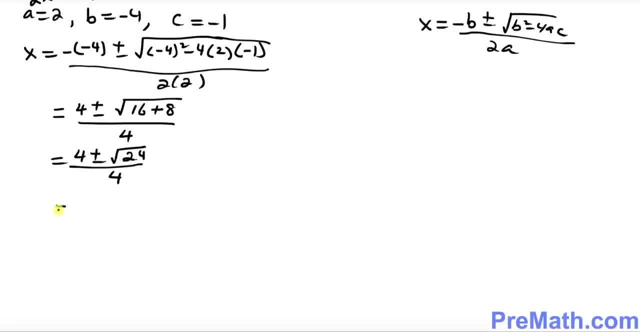 So that could be what happens. So this could be written as 4 plus or minus. the square root of 24 is approximately equal to 4.9 divided by 4.. So we got x equal to this thing. Now, what we're going to do is so we're going to split them up right now along these x. 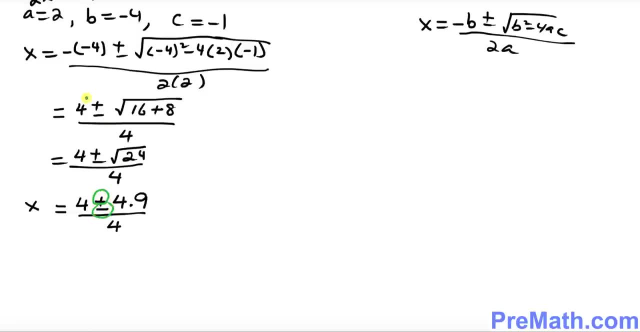 these positive sign and negative sign. So what's going to happen? So then, what we're going to get this way. we're going to get this way. Let's go use this one over here We got four plus 4.9 divided by 4.. And the other way is 4 minus 4.9 divided by 4.. So that's going to give you how much 8.9. 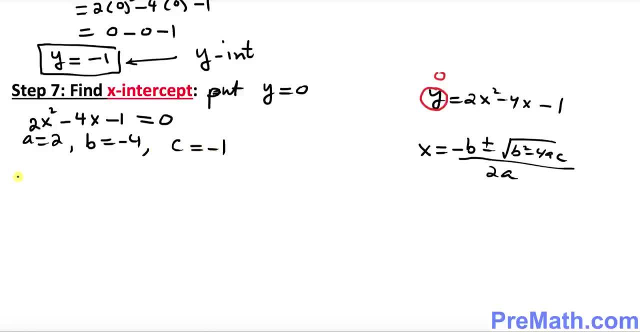 negative 1. Let's plug it in in our quadratic formula to figure out x values. So x equal to minus and negative 4.. What So b is negative? 4 plus minus b square is going to be negative, 4 square minus 4 times. 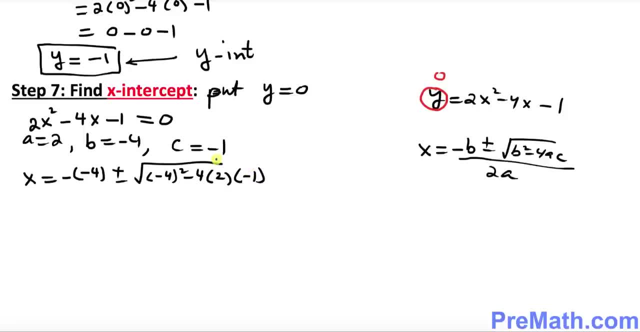 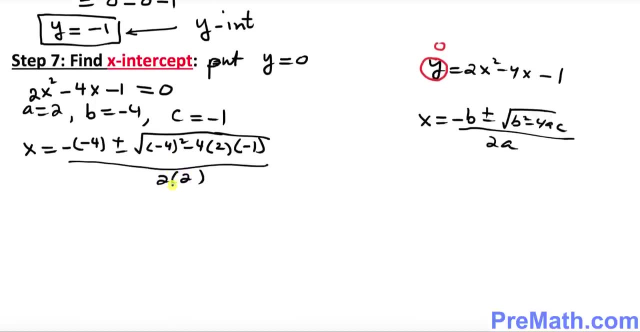 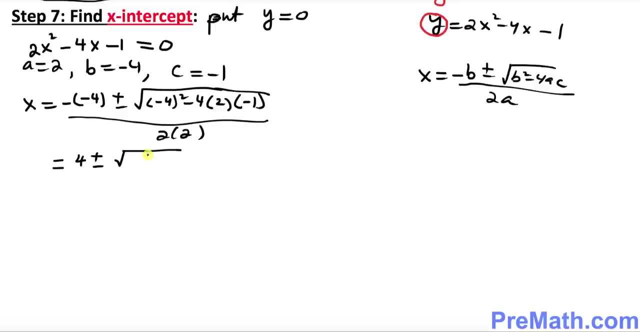 a is 2.. Negative 1, everything is divisible by 2 times 2.. So let's go ahead and simplify that thing. So x is equal to what 4 plus or minus 16 plus 8 divided by 4, let's simply: go ahead, let's put in 4x and minus 4.. All right, So 12 plus 2y. can I get the number 3?? Yeah, Yes, you can, you can. So you can see that I have gotten that right now and you find the jaws are in the whole equation of. 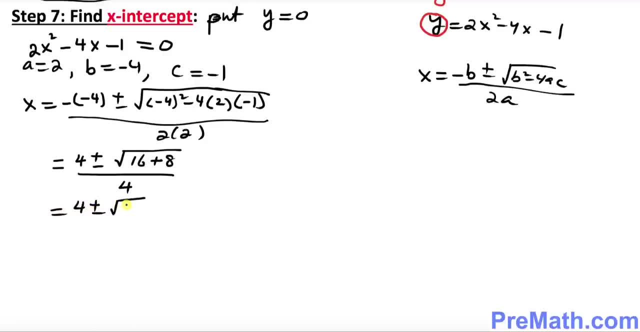 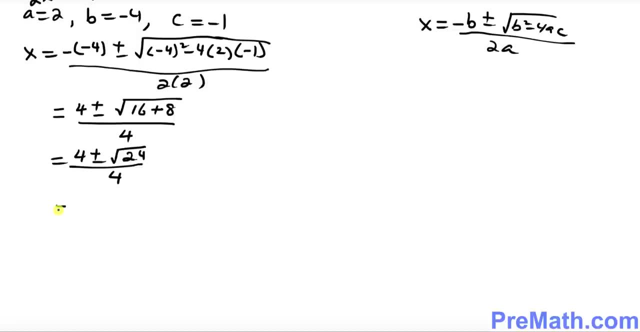 cos there's two lines And that is to verified. I'm going to depict the Superior andенерable 4 plus or minus square root of 24 divided by 4. so that could be what happens. so this could be written as: 4 plus or minus, the square root of 24 is: 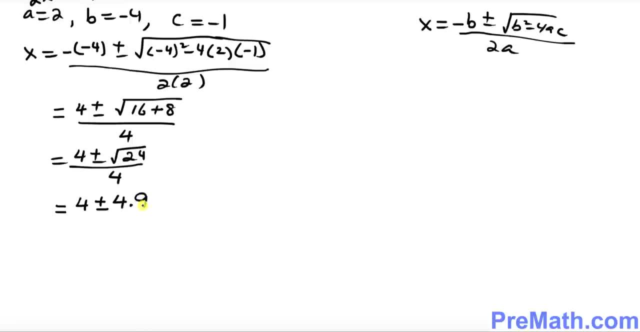 approximately equal to 4.9 divided by 4. so we got X equal to this thing. now, what we're gonna do is so we're gonna split them up right now, along these X, these positive sign and negative sign. so what's gonna happen? so then, what we're? 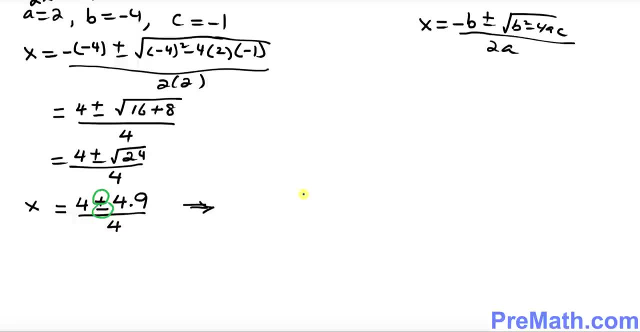 gonna get. we are going to get this way. let's go use this one. over here we got 4 plus 4.9 divided by 4, and the other way is 4 minus 4.9 divided by 4. so that's gonna give you how much 8.9 divided by 4 that. 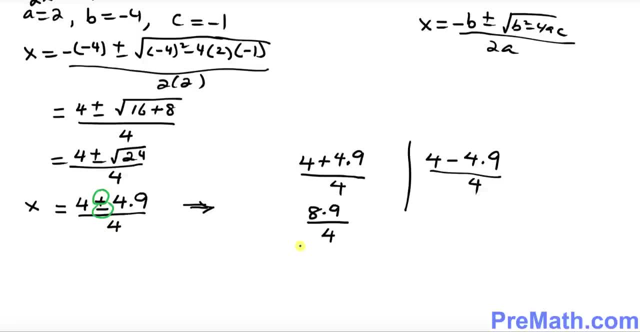 is gonna give you how much? that's gonna give us two point two, three, almost approximately. so one of our X value is this one here. what we're gonna do is we're gonna divide this by 4, and then we're gonna divide this by 4, and then we're gonna divide this by 4, and then we're gonna. 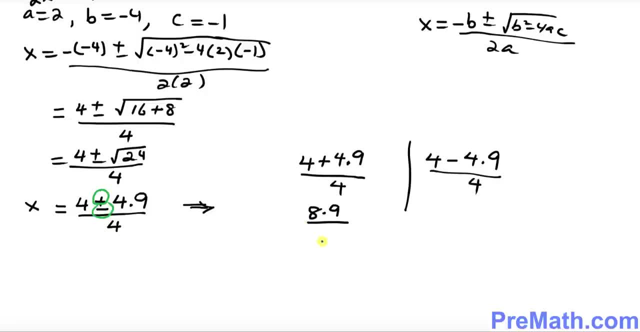 divided by 4.. that is going to give you how much. that's going to give us 2.23, almost approximately. so one of our x value is this one here. what is going to be this one over here? this is negative 0.9 divided by 4. so x is going to be negative 0.23. so these are our two x intercepts. 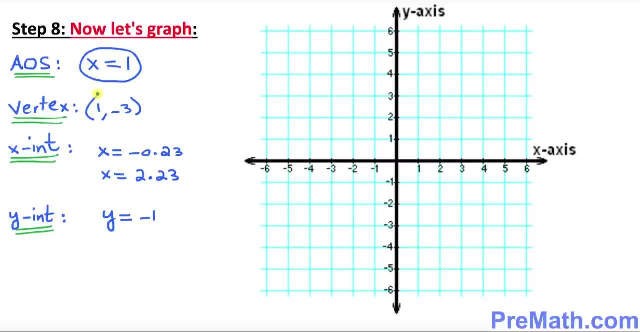 now, in our final step, we're gonna graph this parabola. so in the previous steps we figured out our axis of symmetry was what: x equal to 1 vertex, x intercept and y intercept. so we're going to graph this parabola and we're going to graph this parabola. 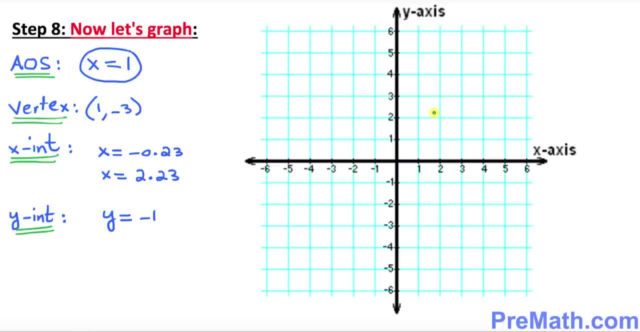 let's put everything together on this XY Cartesian plane, okay, so the very first thing we are looking for: what X is symmetry, X equal to 1, so X equal to 1 is right up here. so this is this is gonna be our. X is off. so this started line. 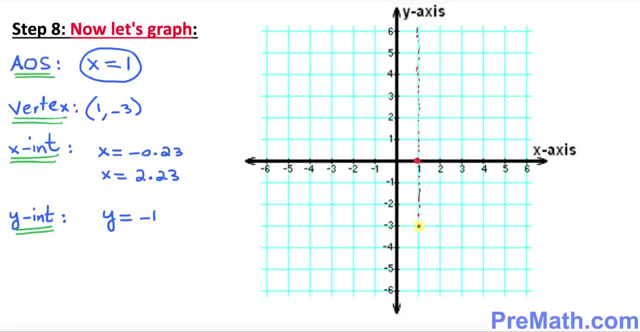 okay, so this is going to be our X is of symmetry is gonna be one much X equal to 1. so this is X equal to 1, right up here. so the next thing is we want to find out our vertex, which is 1 comma negative 3. 1 comma negative 3 is. this is our. 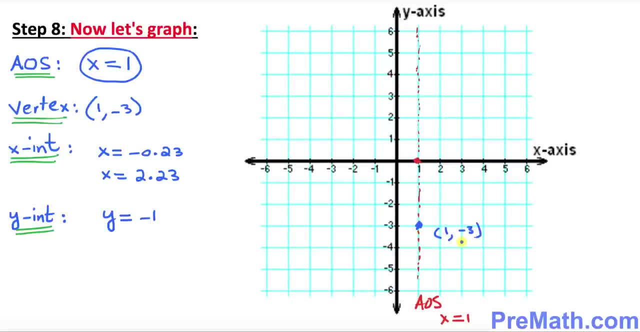 vertex 1 comma, negative 3, which is our vertex, and the next step is we need to figure out what our X intercept, which is negative 2, 3. so that's we're gonna do right now. so negative 0.2, 3 is going to be somewhere here close to the neck. 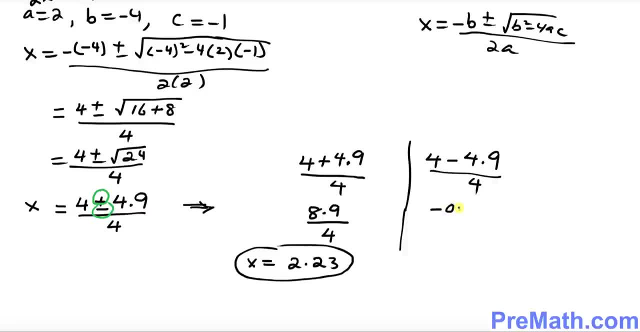 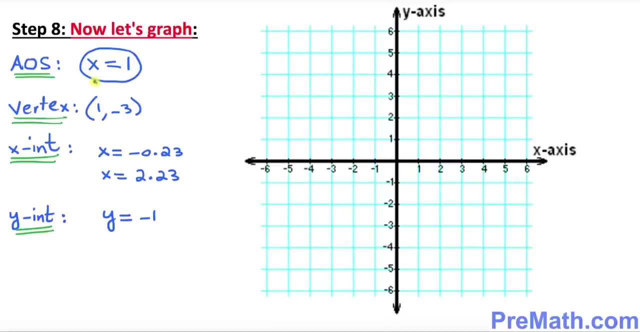 is going to be this one over here. this is negative 0.9 divided by 4, so X is going to be negative zero point two, three. so these are our two X intercepts. now, in our final step, we're gonna graph this parabola. so in the 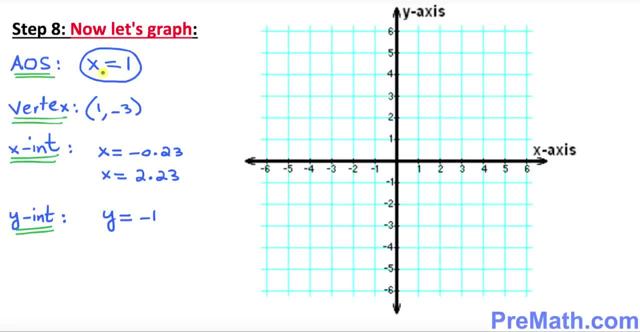 previous steps we figured out. our excess of symmetry was what X equal to one vertex, X intercept and Y intercept. let's put everything together on this XY Cartesian plane, okay, so the very first thing we are looking for, what X is symmetry? X equal to 1. so X equal to 1 is right up here. so this is, this is gonna. 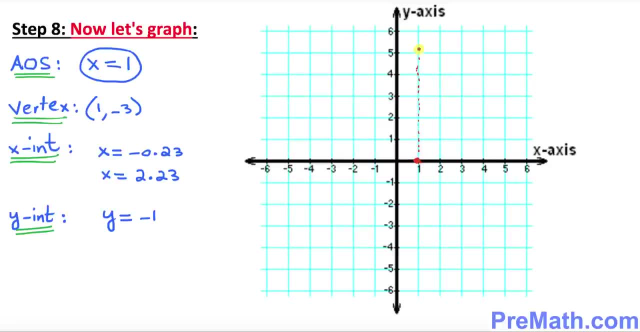 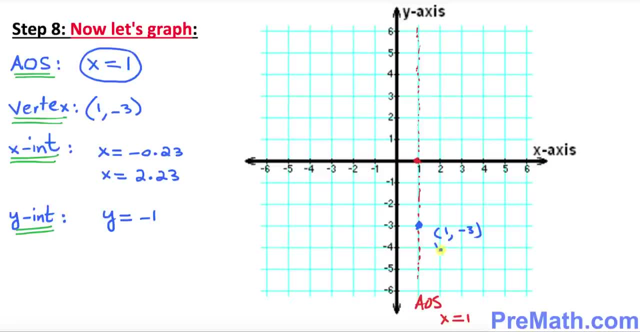 1 comma, negative 3, which is our vertex, and the next step is we need to figure out what our x intercept, which is negative 2, 3. so that's we're going to do right now. so negative 0.23 is going to be somewhere here close to the neg quarter, okay, so this is going to be negative 0.23. and on this,